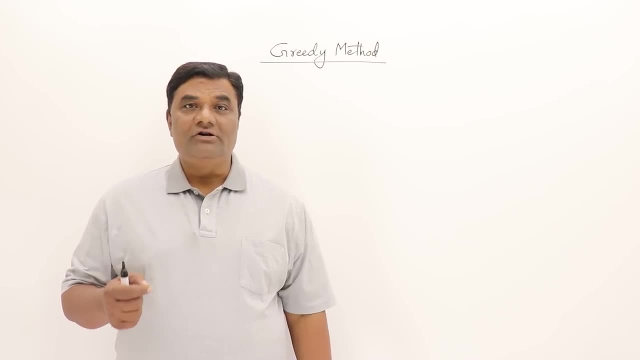 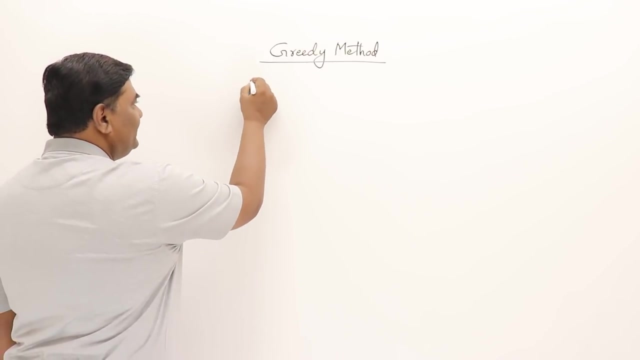 This method is used for solving optimization problem. What are optimization problems? A problems which demands or which requires either minimum result or maximum result. So for this, let us know few terms. I will explain it through an example. Suppose there is a problem P and that problem is: I want to travel from one location A to location B. 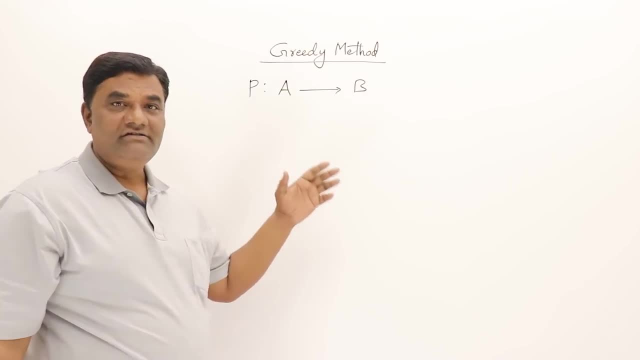 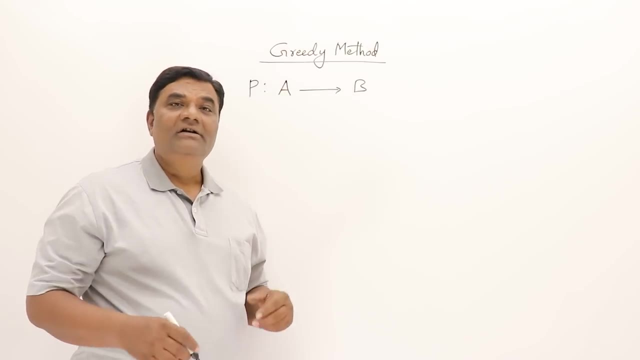 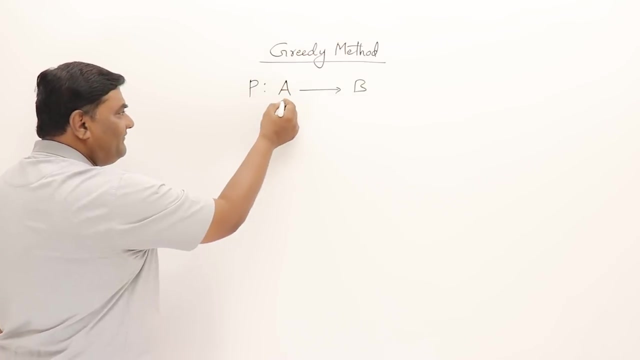 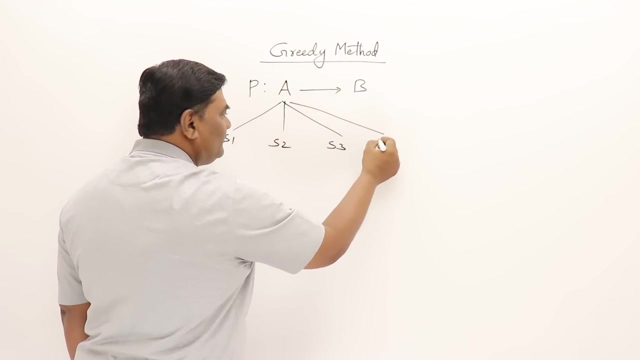 I have to cover this journey. that is my problem. For any problem, I am taking one example, It can be any problem similar type. Now, for this problem there may be more than one solution. Let us say I can travel this by walk- solution 1.. Or I can take a bike- solution 2.. I can take a car- solution 3.. I can go by train- solution 4.. And I can go by flight- solution 5.. And there may be many other solutions. I can take a bike solution 2.. I can take a car solution 3.. I can go by train solution 4. And I can go by flight solution 5.. And there may be many other solutions. 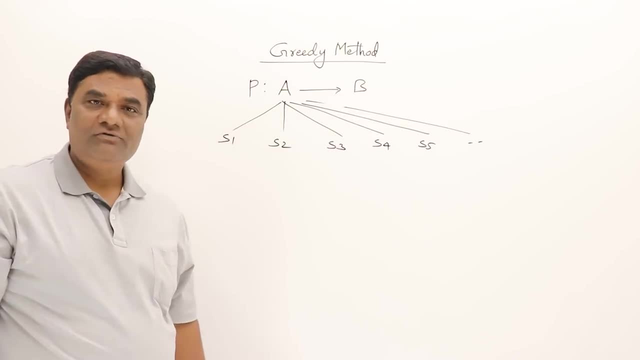 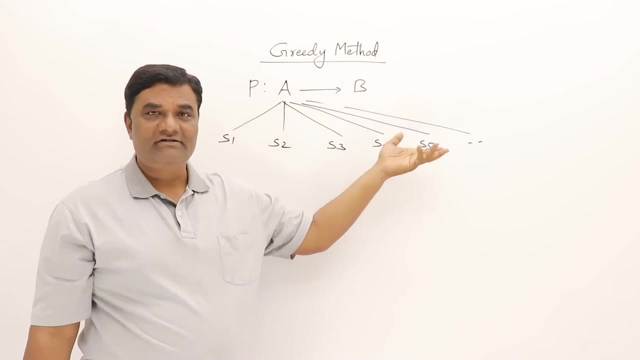 It can give me more solutions. It can give me more solutions. So my problem is to travel from location A to location B and there are many solutions. You go like this, or take this, take this and go there, But there is a constraint in a problem. I say that I have to cover this journey within 12 hours. 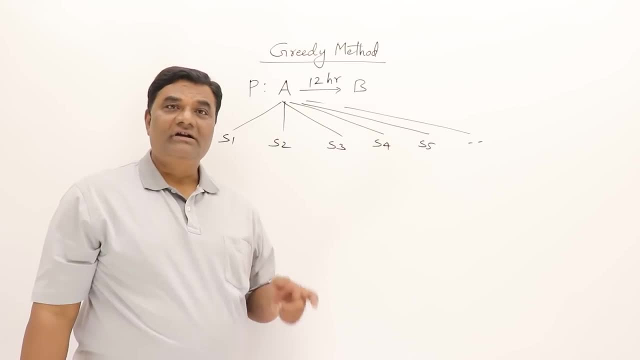 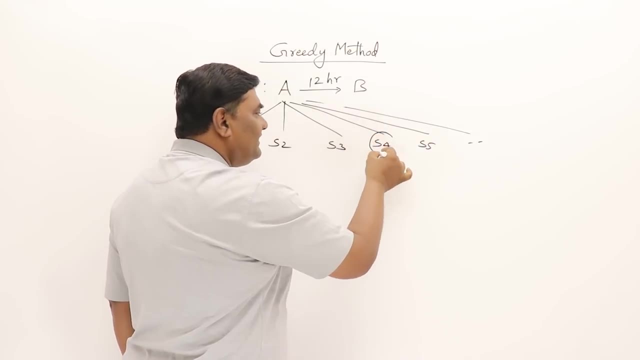 This is the condition constraint, So suppose I cannot cover it if I go by walk or by car and so I have to cover this journey within 12 hours. This is the condition constraint. I can cover it only if I go by train or flight. 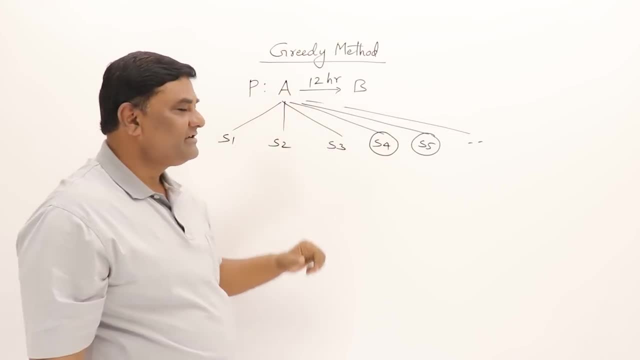 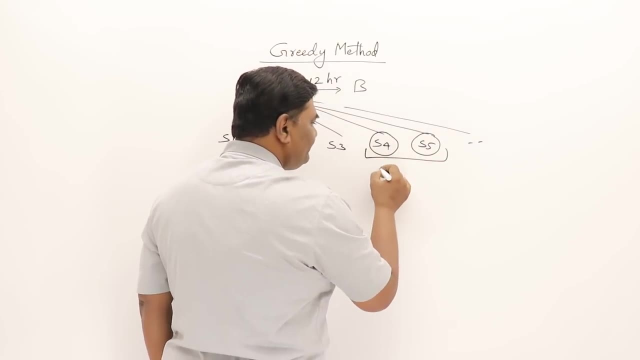 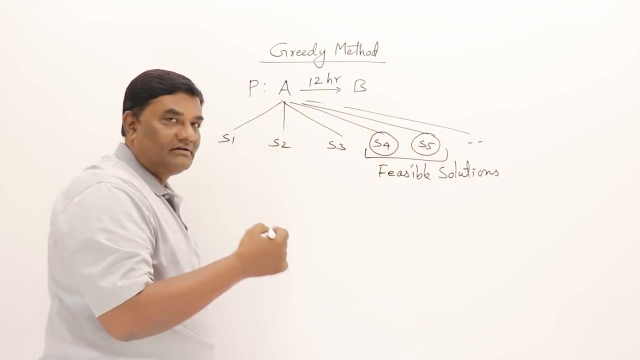 Now for a problem. there are many solutions, But these solutions which are satisfying the condition given in the problem, then this type of solution becomes feasible solutions. This is the meaning of feasible solution: A solution which is satisfying the condition given in the problem is feasible solution. 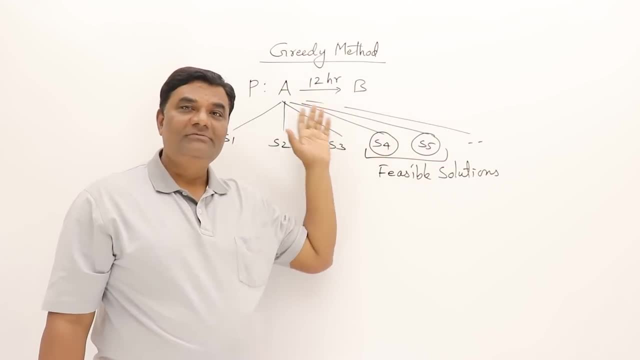 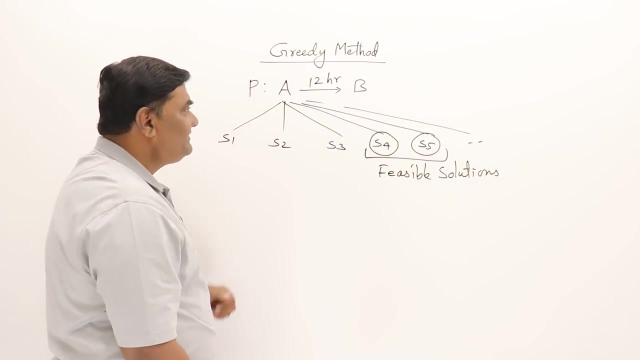 Though for a given problem there may be many solutions, This is feasible solution satisfying the constraint. Commonly we use the term: is it feasible or not Feasible? in the sense what? satisfying our constraints or not, limitations or not? Next, if I say that I want to cover this journey in minimum cost, 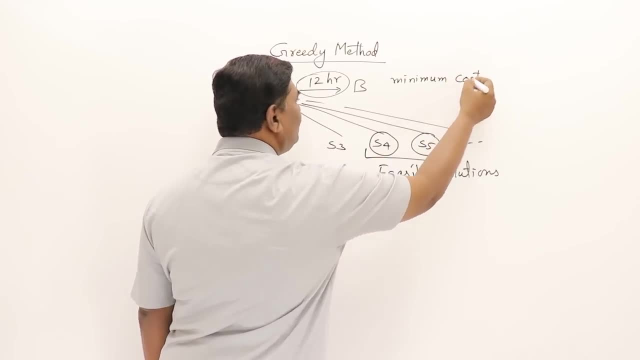 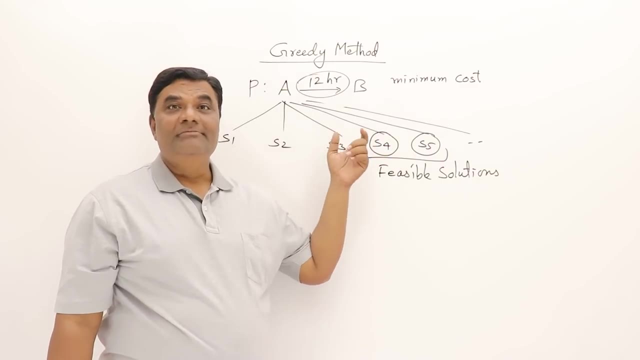 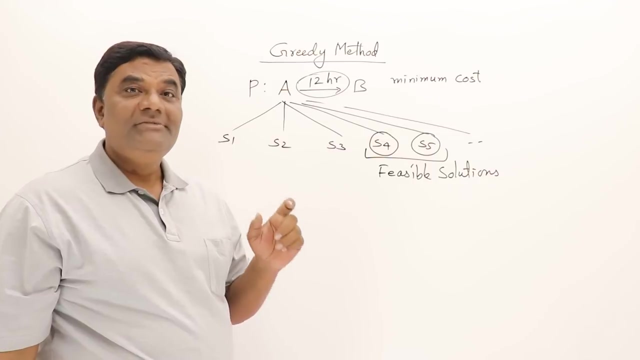 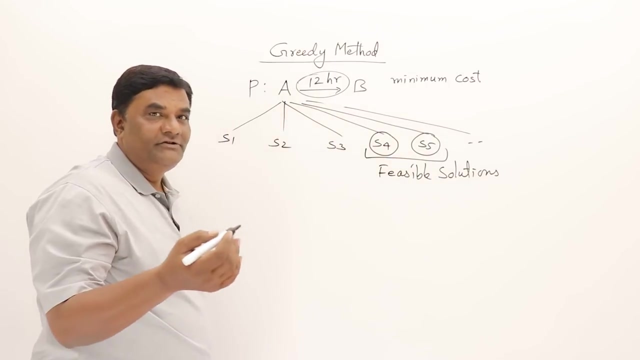 Minimum cost. I want to spend as much as less possible. Then this becomes a minimization problem. So now, as the problem demands, a result should be minimum, Then it is a minimization problem, Right, Then, out of these two solutions, one of the solutions may be taking minimum cost. 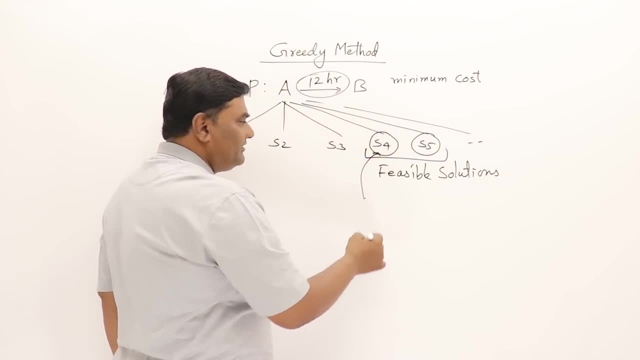 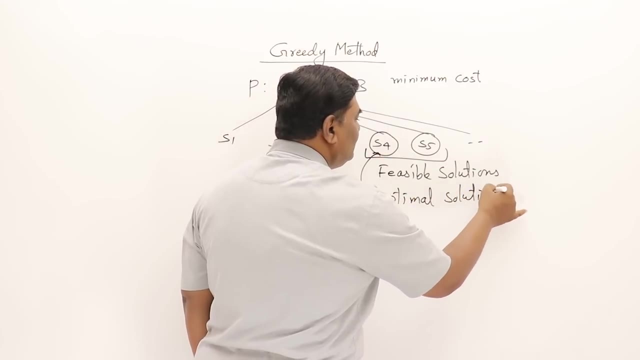 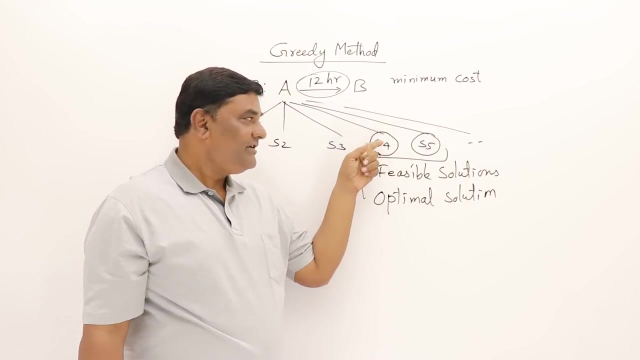 Suppose, by train, if I go, this is minimum cost. Then this is called as Optimal solution, A solution which is already feasible and also giving me minimum cost. That is best results. That is best for me. Minimum is best for me. 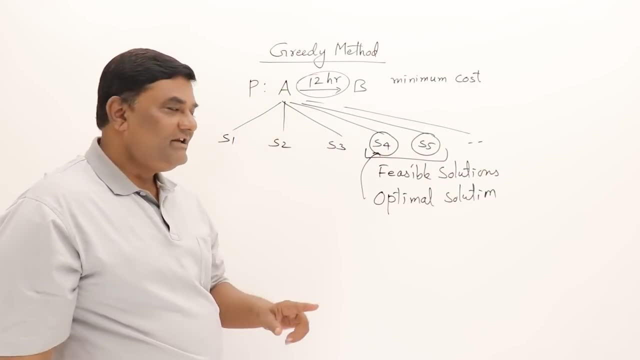 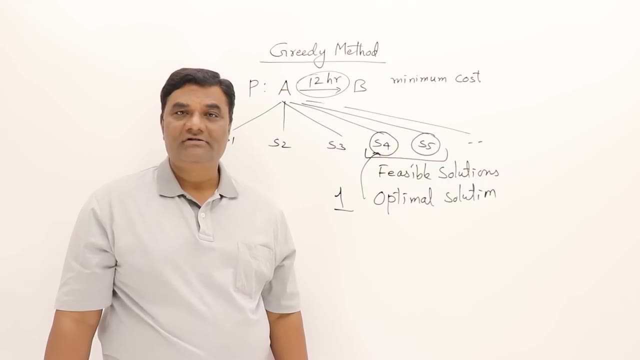 Then that solution is called as optimal solution And definitely for any problem there can be only one optimal solution. There cannot be multiple optimal solutions. That means there can be only one minimum cost. Minimum can be only one. There can be more than one solution. 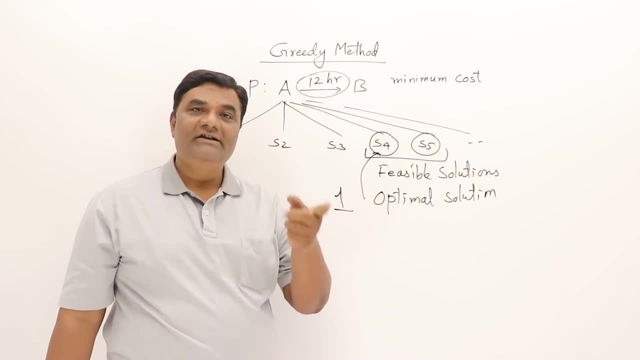 There can be more than one feasible solution, But there will be definitely only one optimal solution. This problem requires minimum result. Some other problems may require maximum result. So if a problem requires either minimum or maximum results, Then we call that type of problem as. 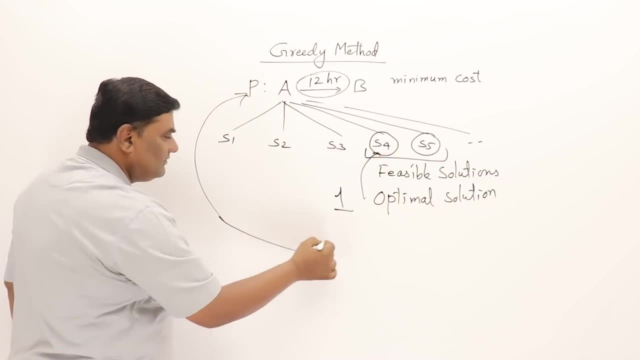 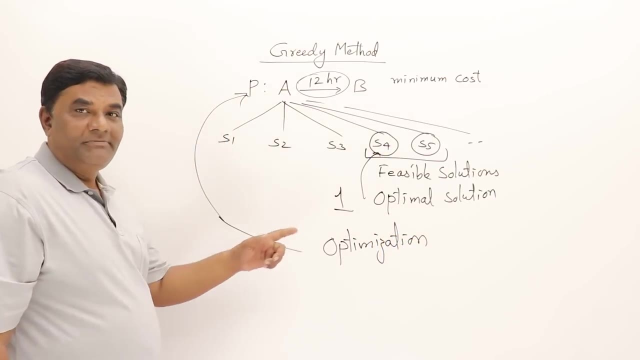 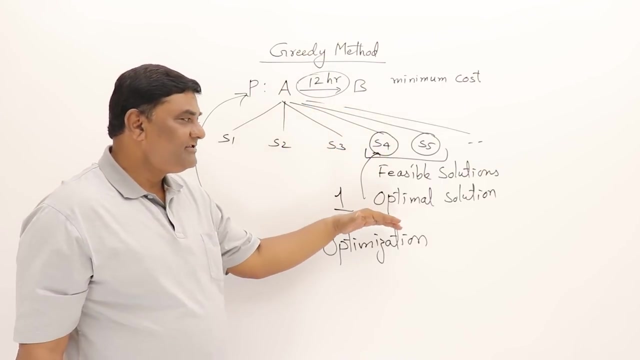 Optimization problem. Optimization problem is one which requires either minimum result or maximum result. So let us briefly look at the terms once again. Feasible solution means a solution which is satisfying some constraint. Optimal solution means which is achieving the objective of a problem. 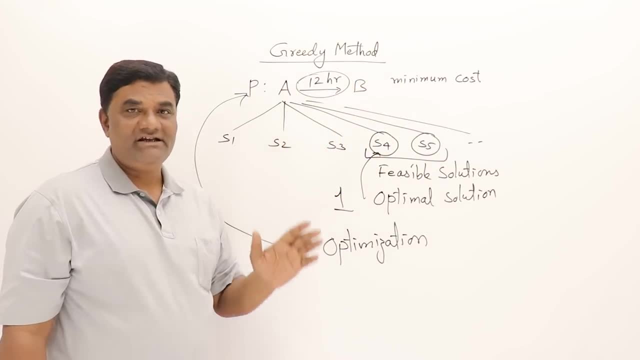 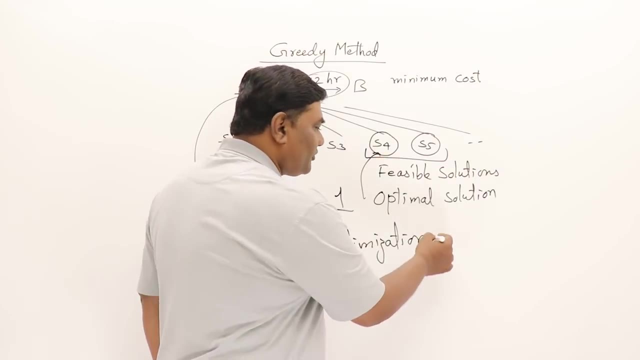 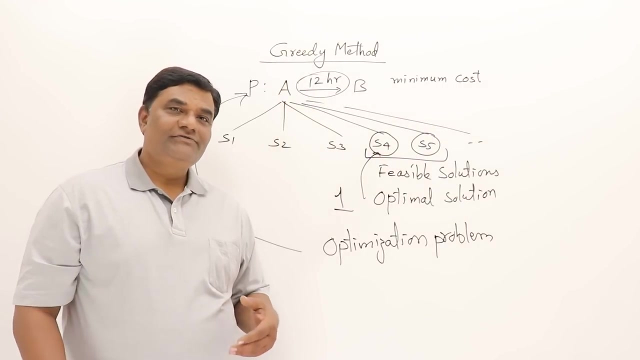 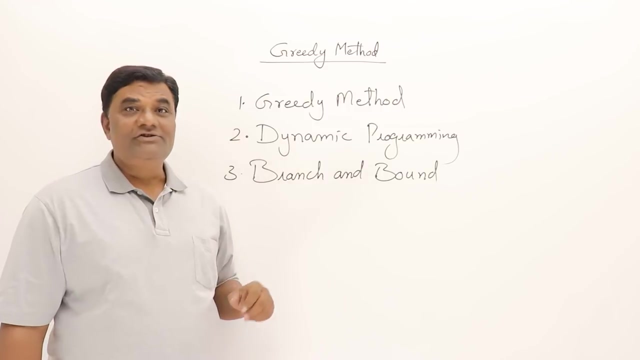 Satisfying the objective of a problem That is either minimum result or maximum result. A problem which requires a minimum or maximum result is a optimization problem, So greedy method is used for solving optimization problems. These are the strategies used for solving optimization problems. 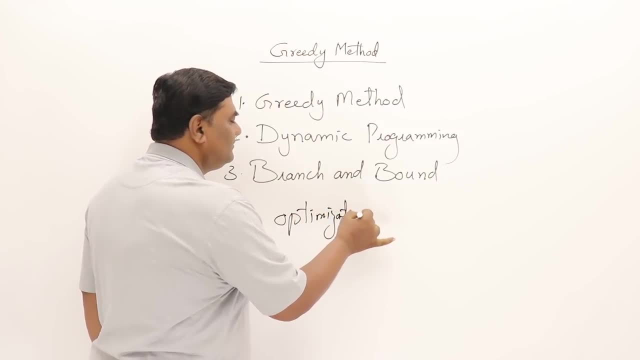 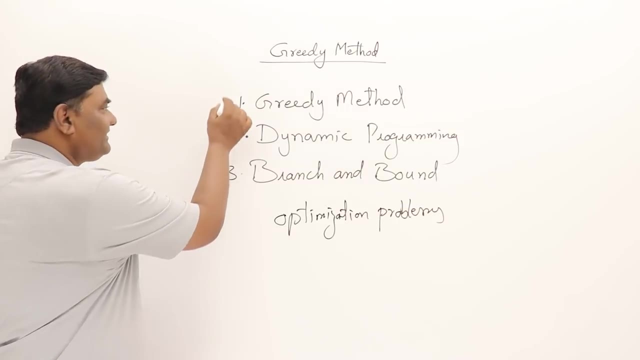 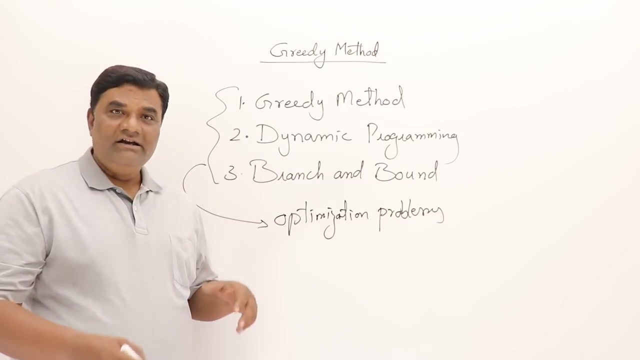 These three methods are for solving optimization problem. The approach is different And every problem, whichever, requires optimal results. Some may be suitable here, Some may be suitable here. This strategy can apply on it, Or some this strategy can be applied, Or some for some problems. 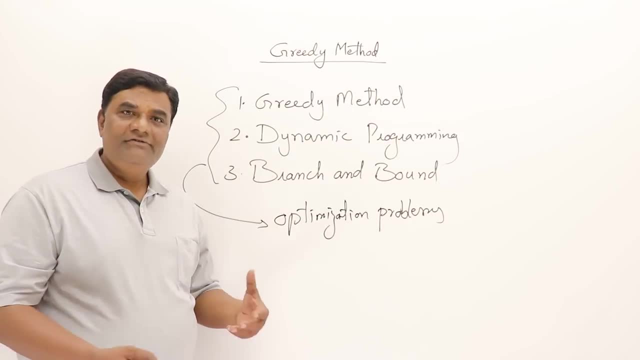 All three strategies can be applied on them. So we will learn all these strategies through problems, one by one. Now we are going to cover this greedy method. We will start with greedy method. We will understand what greedy method says. What is the approach? 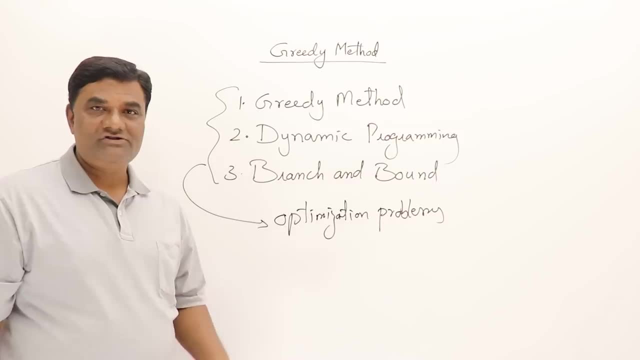 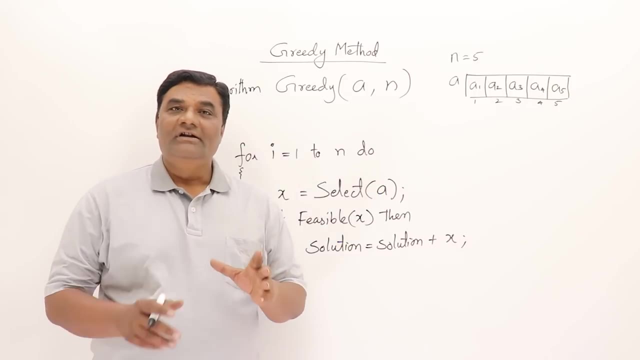 So next I will tell you about greedy method. What is its approach? Here is the general method of greedy. I have written an algorithm, See. greedy method says that a problem should be solved in stages. In each stage we will consider one input from a given problem. 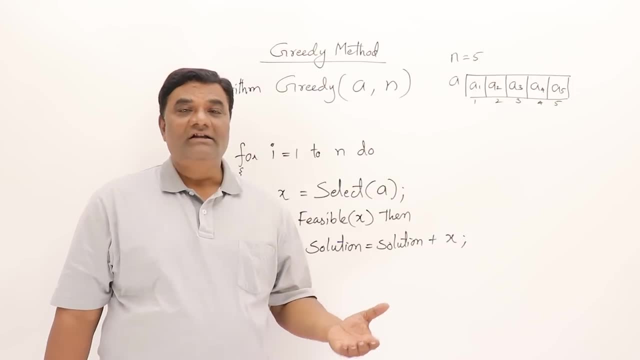 And if that input is feasible, Then we will include it in the solution. So by including all those feasible inputs We will get an optimal solution. So in stages we will, each time we will pick up our input And we consider it, And if it is feasible, 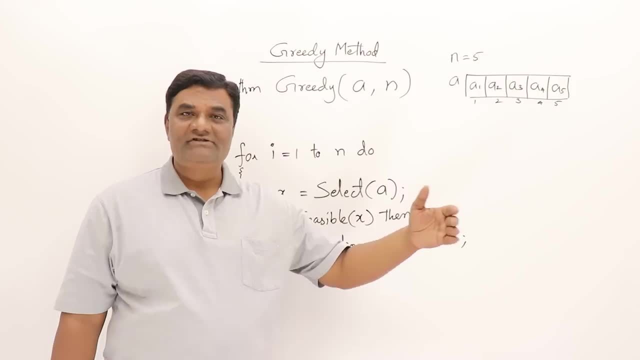 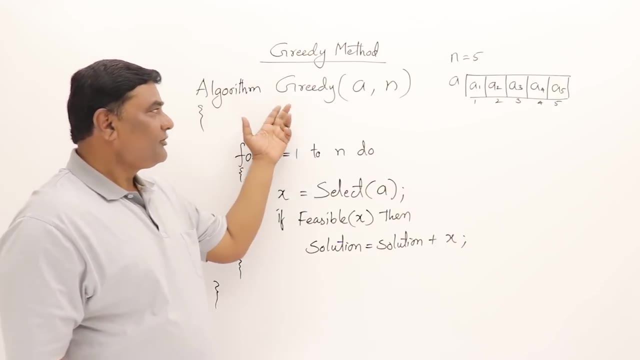 We will include it And like this, if we follow this procedure, We will get the optimal solution. So here a general method is given. If a problem is given And that problem is having an input of some size, And n is the size, 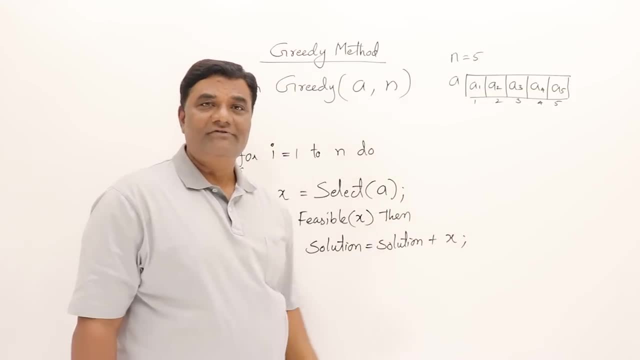 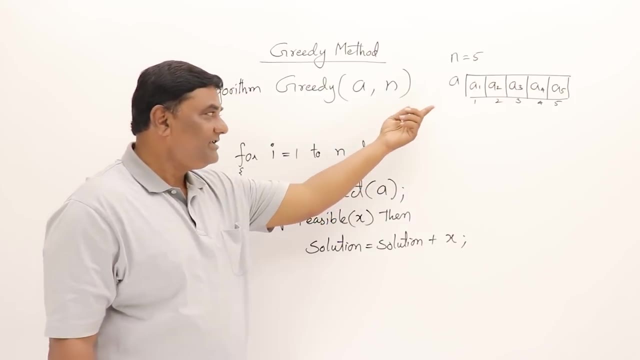 And it is having some data, Some values, Input values. Now it will go through all those input values from 1 to n, And each time it will select something from a And call it as x, If that x is feasible. That is one input. 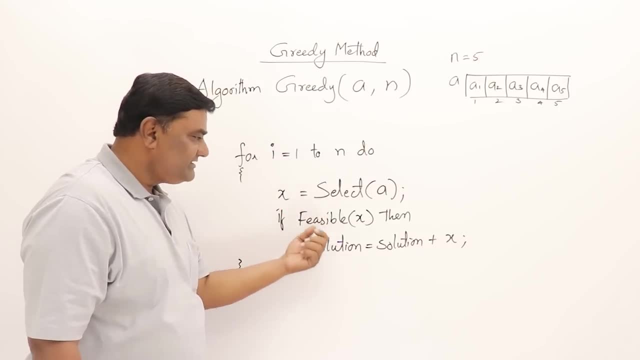 One by one. it will pick up the input And that input, if it is feasible, It will include in the solution. If it is feasible, It is included in the solution. So this comes under, if This is the general method, Now I will explain you through example. 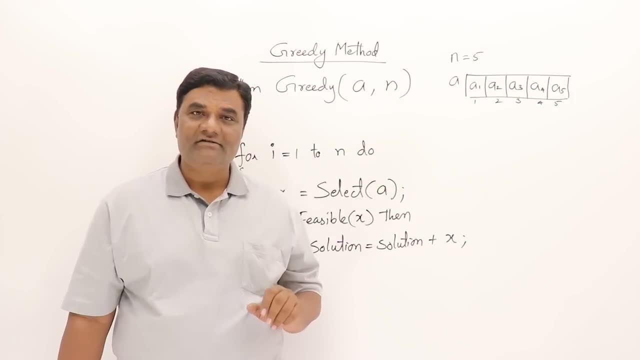 The approach of greedy method Is that, Suppose, if you have to buy a best car, Best car, Best car in the sense In terms of features, You want a best car, Optimal, Optimal, Okay, The cost will be maximum, definitely. 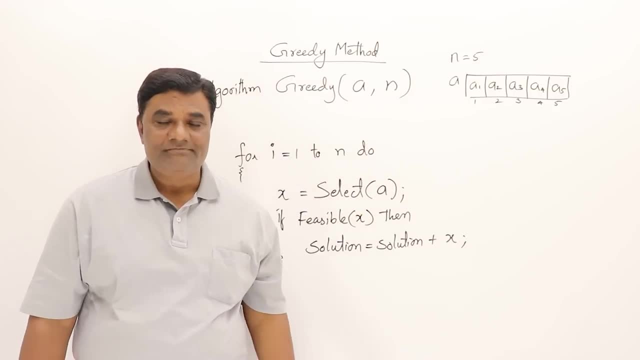 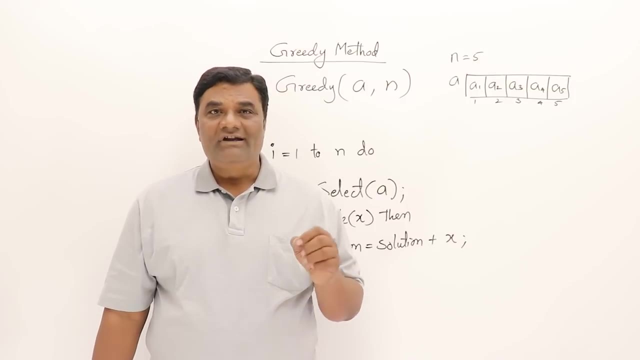 So, but you want optimal. Optimal in the sense In terms of features. Now, how do you choose a best car? How do you choose a best car? So one method is: You should look at all the brands And all the models of cars available in the world. 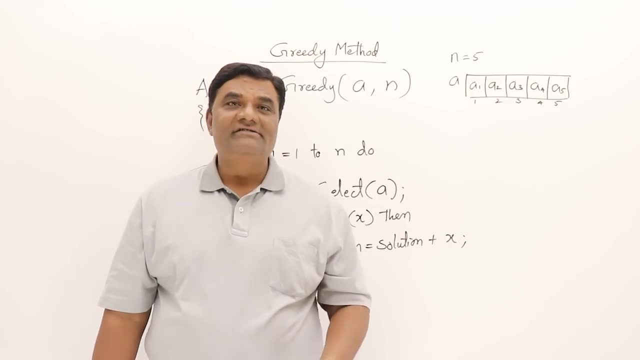 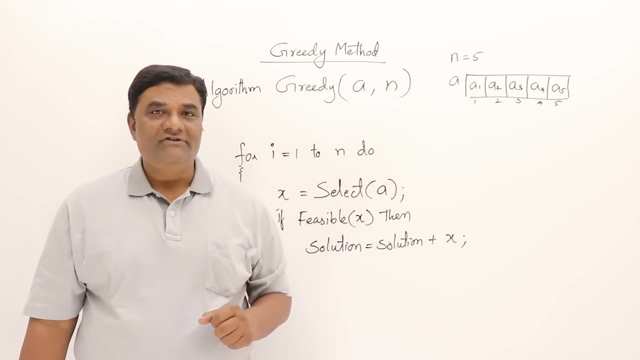 Or at least in your city. Then you can say that I have checked all the cars, Then I have selected the best car. This is one approach for solving a problem. The problem is to buy a car. This is one method. This will be very much time consuming. 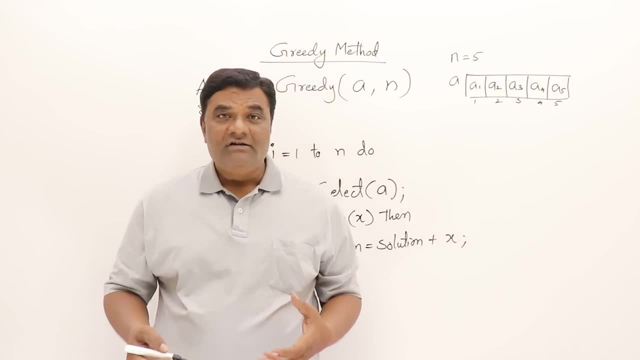 You have to check each and every brand And every model. See, the cost may not be a thing Sometimes. otherwise car May be better than costlier car. So, checking with the features, And you are deciding that This is the best car. 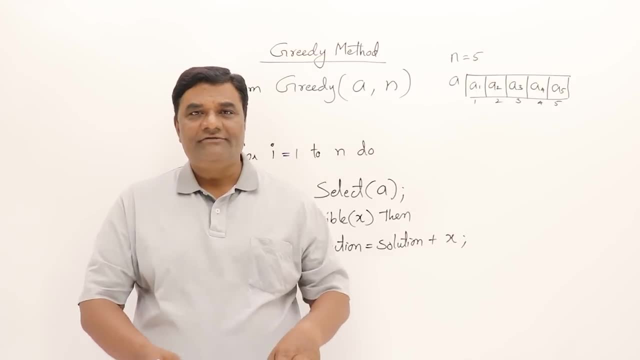 So, but actually, what is the method we follow? We first of all sort out the brands And we say that we don't want in this, this We want. Let us say, you are selecting a brand that is Toyota Or Hyundai, Right. 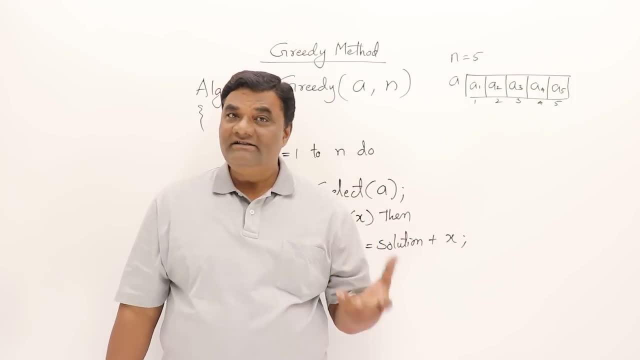 Okay, You are saying that these are the best brands for you And in these brands, Then again you will select the top models, Right, So you are not looking at the lower models. So again you have sort out. Then again you say that in this top model, 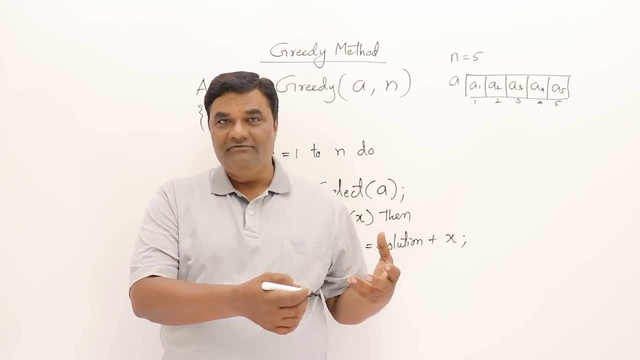 The latest release car, Or the well known car, Well tested car. You are picking up that one And you are saying that this is the best one. Is it really the best one out of all the cars in the market? For you, it is the best one. 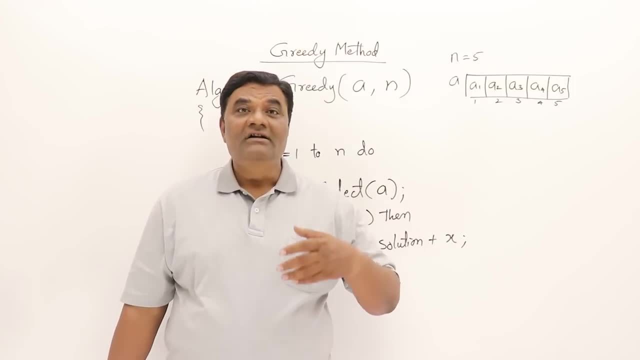 So what is the approach you adopted? You have adopted a greedy approach, So you have your own method of selection And based on that selection method, You got some result And you are saying that this is the best result. That's how it is greedy. 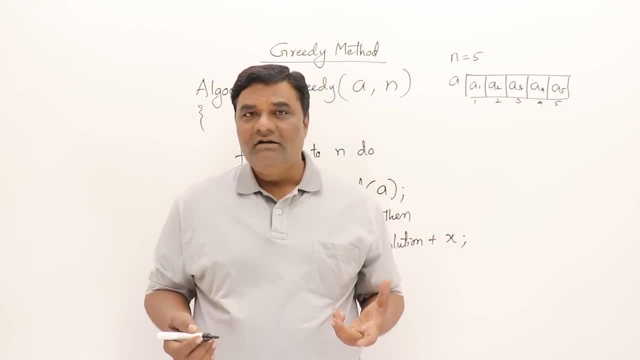 And definitely, when you do this, You will be picking up the best car, So you don't have to waste time in checking all the cars Available in the city, Available in the market. So that's it. So, without checking all of them, 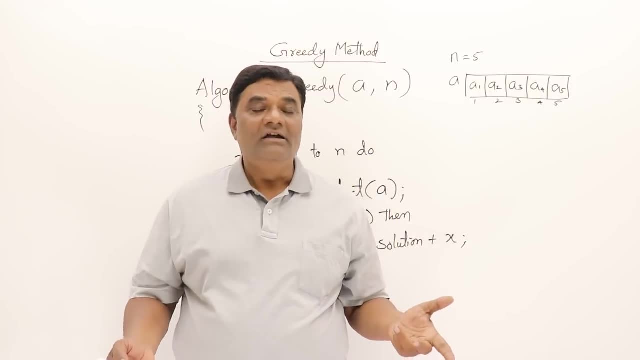 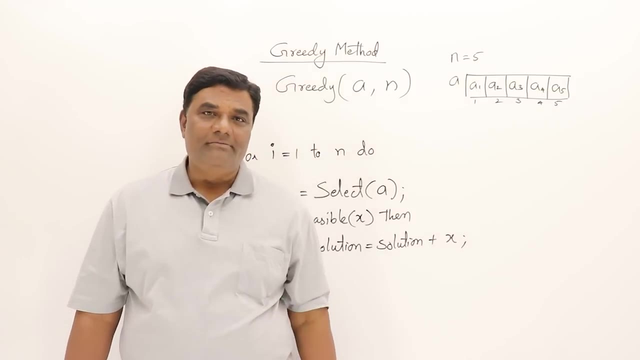 You say that You select few And say this is the best car. No doubt That is the best car, But the approach you adopted is greedy. I will give you one more example. Suppose you are running a company And you want to hire some people. 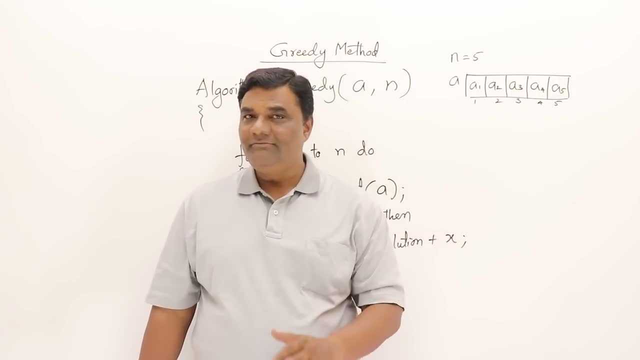 So when you have given an ad, Some thousand people came to you for the interview. Now you will conduct some type of test, Like first you conduct return test And then you have a technical test Or group discussion. Like that you will have various phases of test. 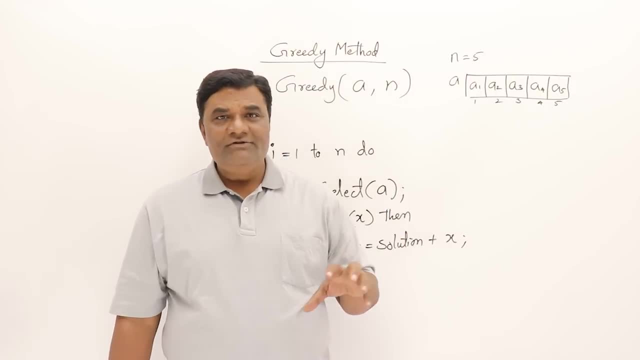 And you will filter the people And finally you select one person And you say that this is the best person out of those thousand. Is he really a best person? Yes, according to your procedures, It's a best person. What was your selection procedure? 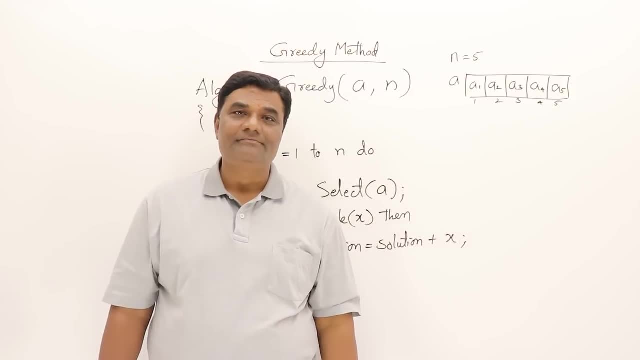 Based on the selection procedure, He is the best person And, yes, You have got the optimal solution. So the approach is greedy. Many students complain that I was better than him And he got selected. They think like that, But really the person who got selected is the best one. 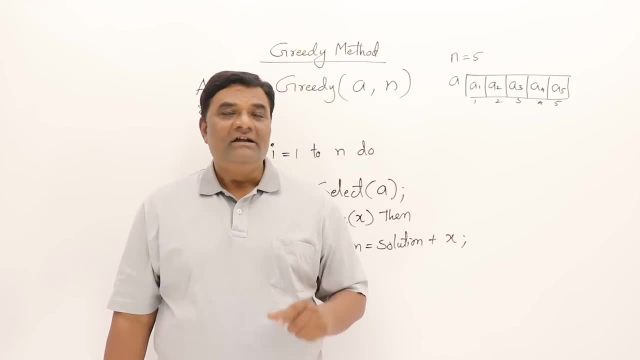 Definitely So, the approach that you are adopting. Now I will tell you: If you are selecting one person out of thousand, Then for all, you should give a chance for return test. For all, you should give a chance for group discussion. For all, you should give a chance for technical interview and HR interview. 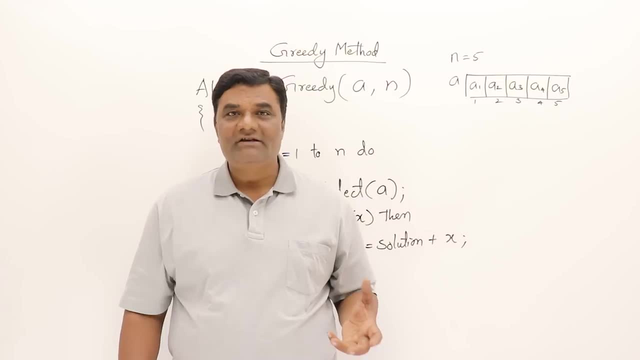 Then pick up the best one. This will be very time consuming and costly process. We don't do that. We simply filter the people and select the best one. This approach is called as greedy approach, So we have our own methods of selection.